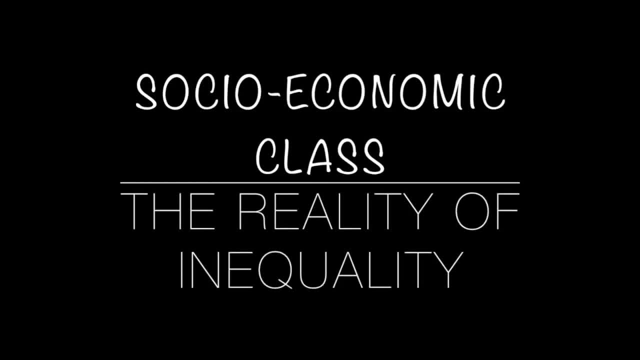 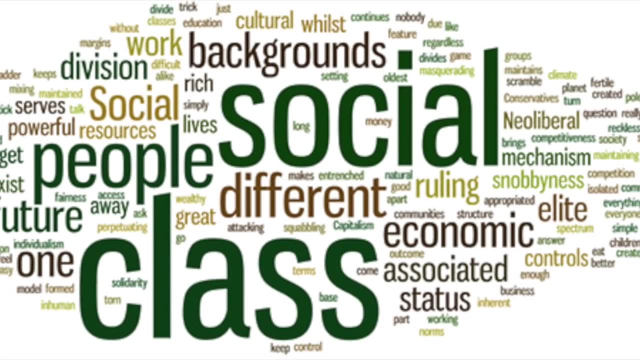 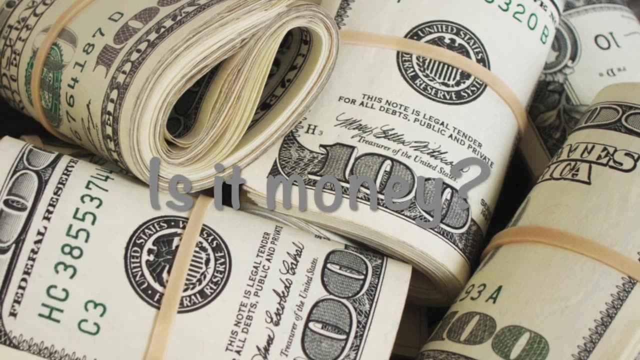 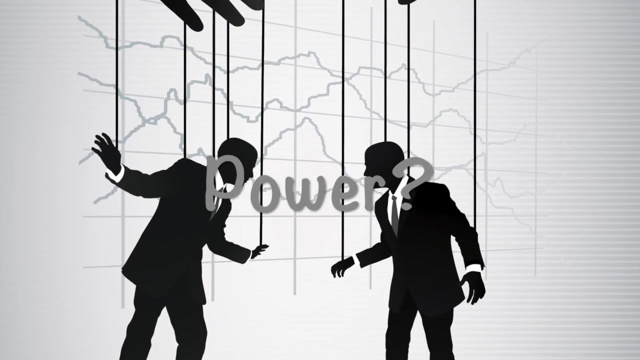 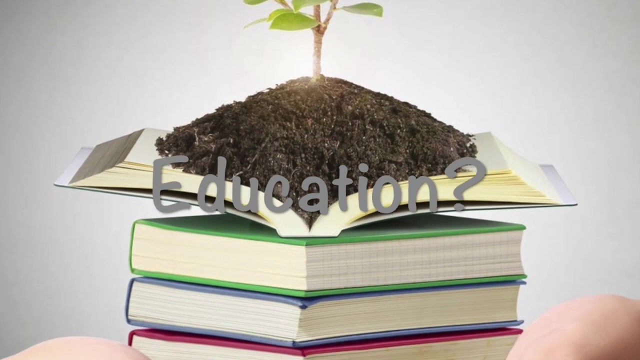 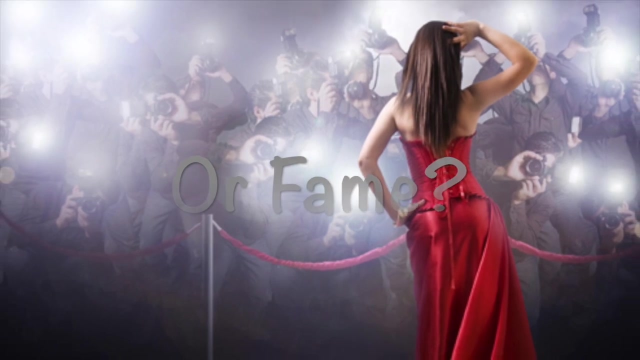 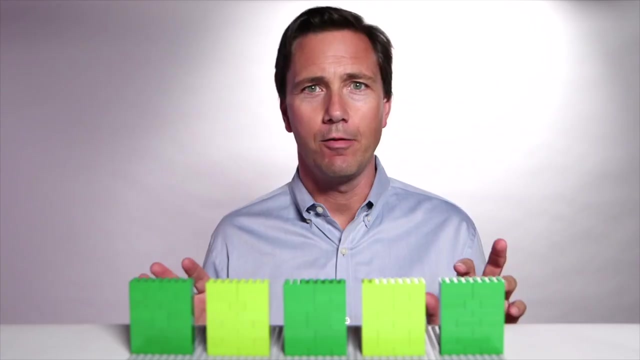 Ask yourself a question: What is social class? What comes to your mind when you think of social class? We're going to talk about inequality and opportunity in America. Let's start by dividing the population up into five equally sized slices. If you're boring, like me, you might. 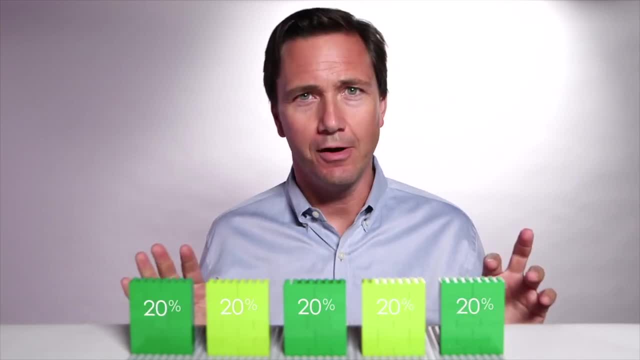 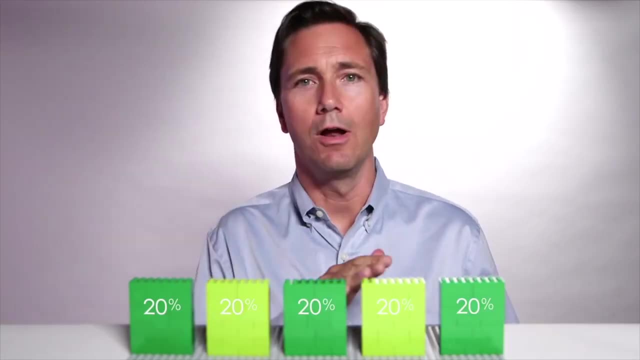 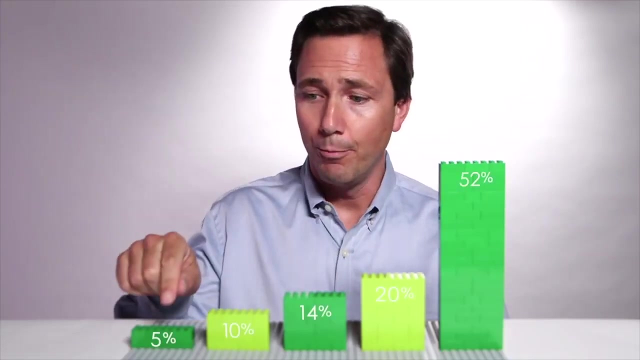 call them quintiles. In an absolutely equal society where everybody had the same amount of money, each fifth of the distribution would get a fifth of the money. It would look like this. Of course, that's not how it is In the real world. the bottom: 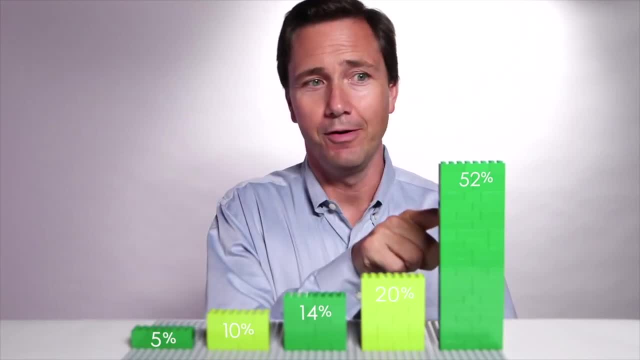 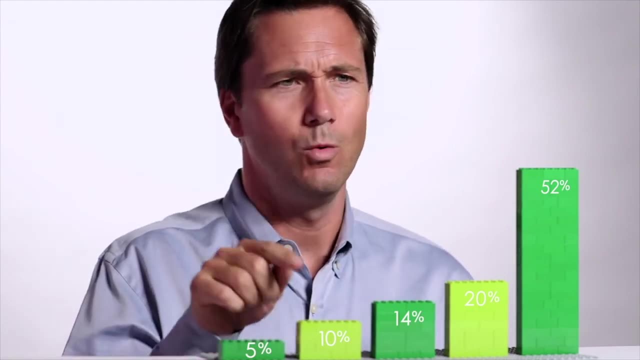 quintile. the bottom fifth gets 5% of the money and the top fifth get more than half the money. But I think in terms of fairness, and certainly in terms of American fairness, the question is less what's the gap between the bottom and the top, and it's more what? 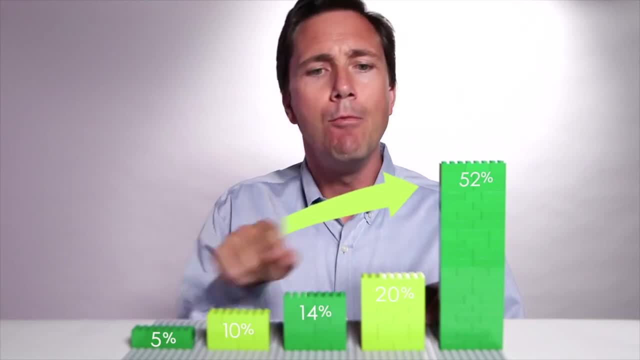 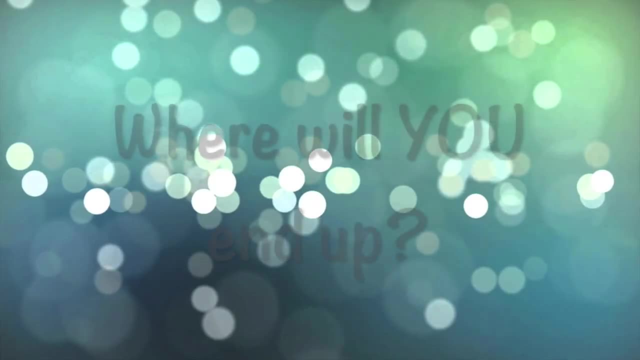 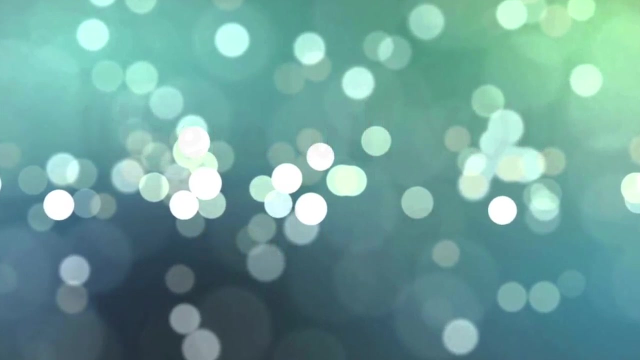 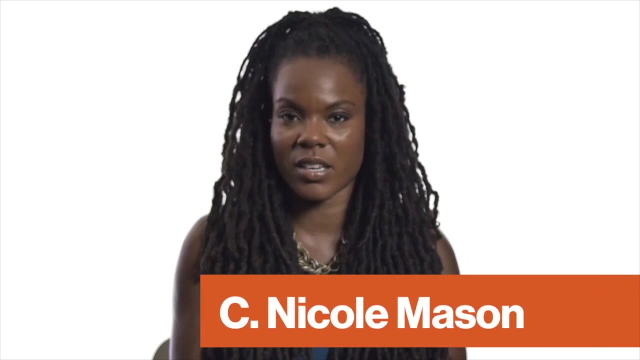 are your chances of making it from the bottom to the top? How mobile is society? How far does where you're born on the ladder? How does that affect where you end up on the ladder? We're not talking honestly about what it really takes to get from poverty to the middle class. 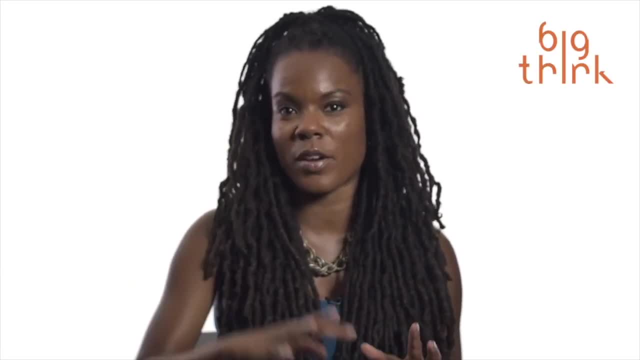 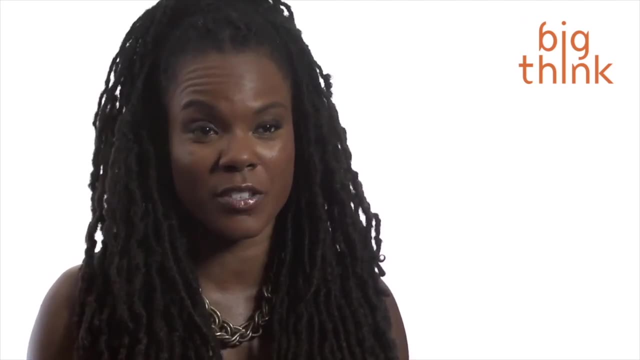 For example, we know that only 4% of people who are born into poverty will ever make it to the upper middle class. We know that only 4% of people who are born into poverty will ever have middle-class success. What that means is that 96% of people are not making it out. I think we're being dishonest. 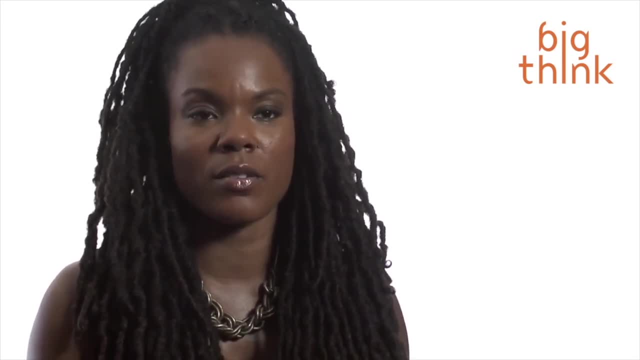 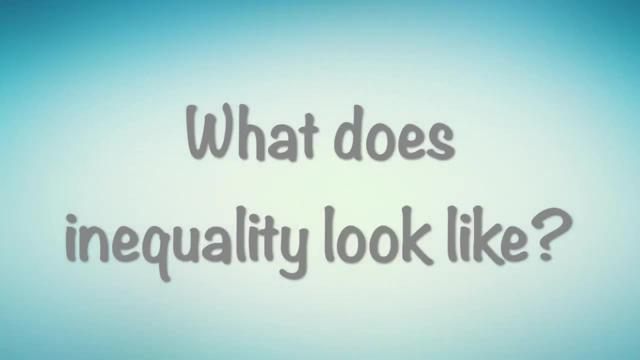 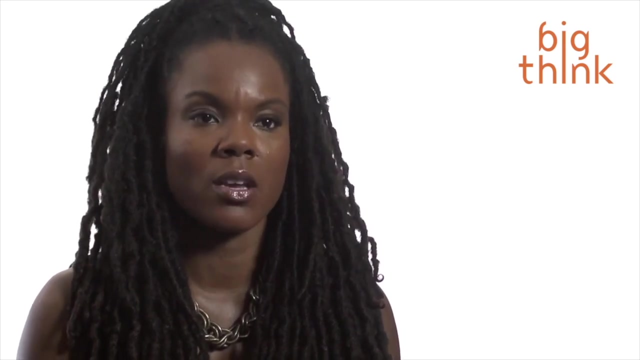 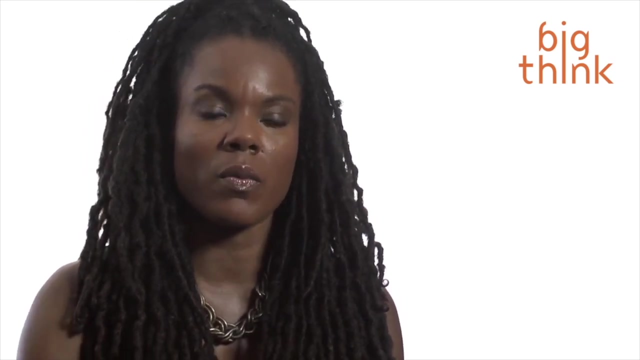 when we say everybody has a fair and equal chance of achieving the American dream. When people think of poverty, they think about money and resources and cash, But a big part of poverty is the lack of social connections. What we know is that those social networks and connections are really powerful in terms 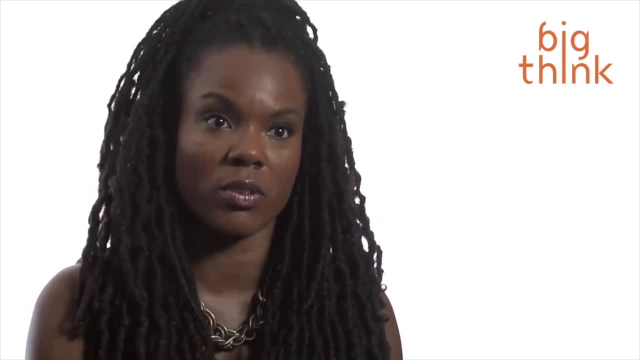 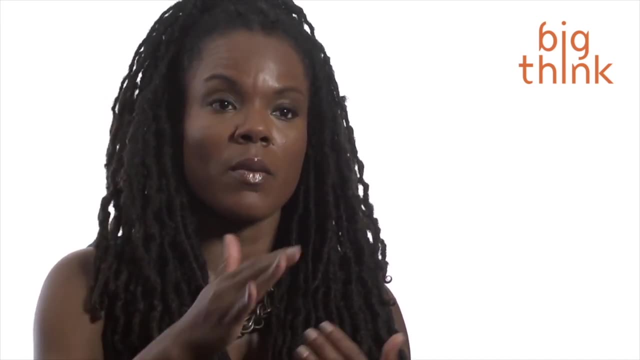 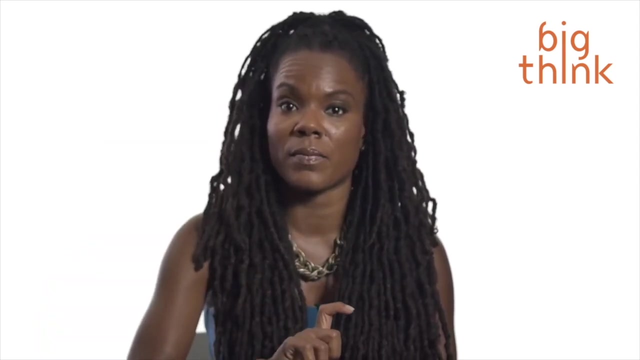 of helping people to navigate complex institutions and structures For poor people, those social networks are often missing. When we talk about bridging from poverty to the middle class, social networks and social capital are really important to making that leap, So I think we need to16. 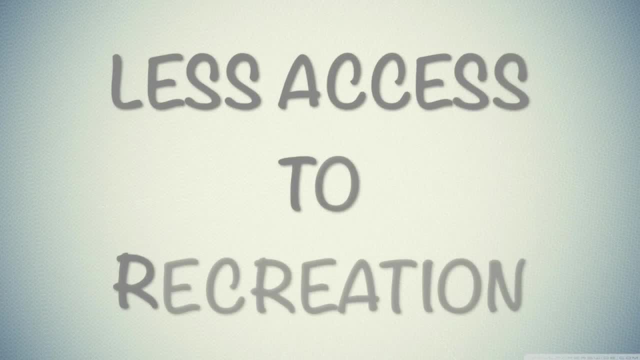 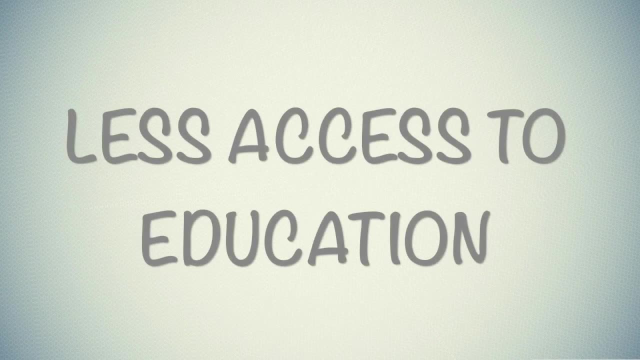 make sure that we have a working culture, inclusive culture. What we have is too many puzzlesclamation boards and illegals to be able to drag. No 허 Where people, when it comes to these VC calls, Niall Yoakam, can do inm allez bien. statements, do them a favor and speak about the conversations we need to have with our community. So for both sets of letters, I think the rest of the world's understanding of how Rambo works is really important, and it is the right thing to say to Хэйлойн. 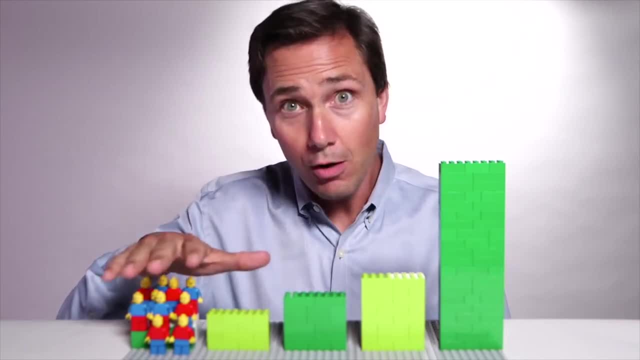 Wagner, Our alors 🚎🚎🚎 🚕🚕� немоном me is working together, working together with. I wish I had a App Store and trophies and windows of small businesses that should be owning for the full cost of living. 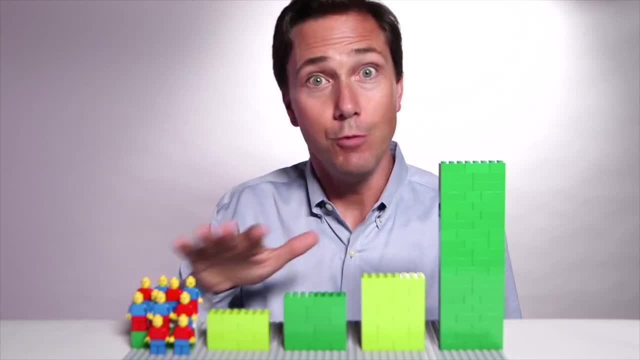 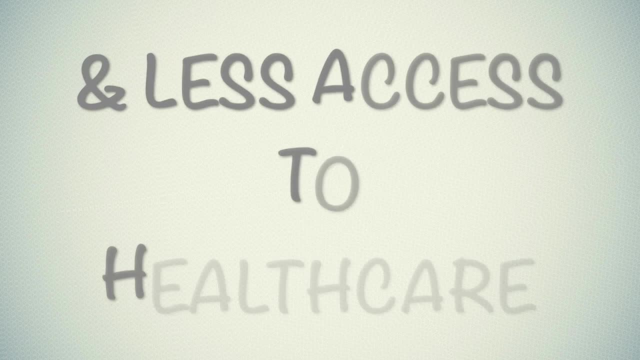 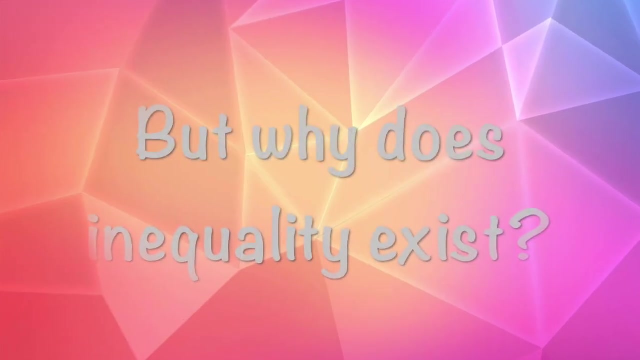 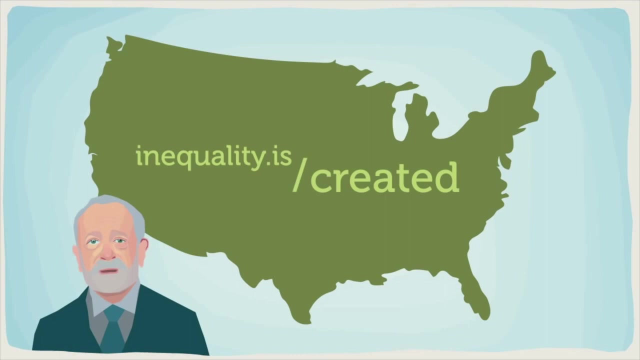 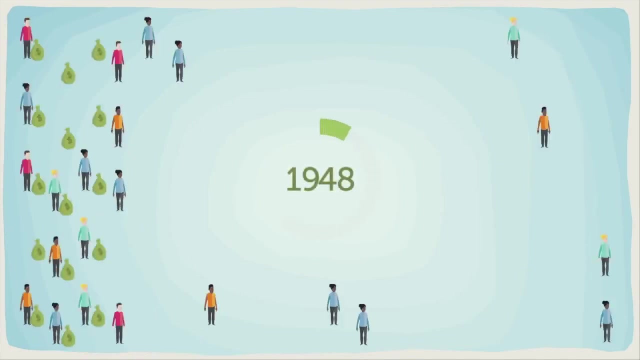 If you manage to get a four-year college degree, it transforms your chances of moving up the income distribution. Go to college. The recent past has seen greater economic inequality in America than at any time since the Great Depression. In the three decades after World War II, American incomes grew quickly and equally. 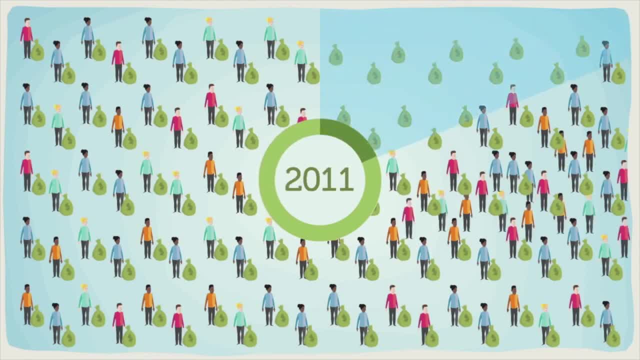 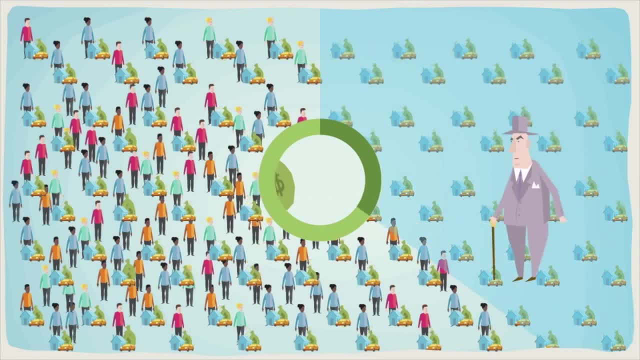 But starting in the late 1970s, things began to change. Today, 1% of Americans are taking home nearly 20% of the country's total income and own more than 35% of America's wealth. And it didn't happen by accident. 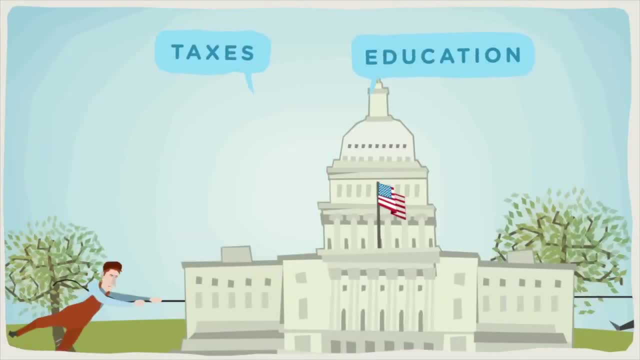 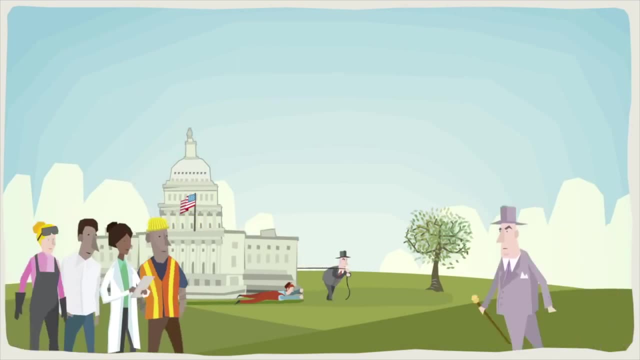 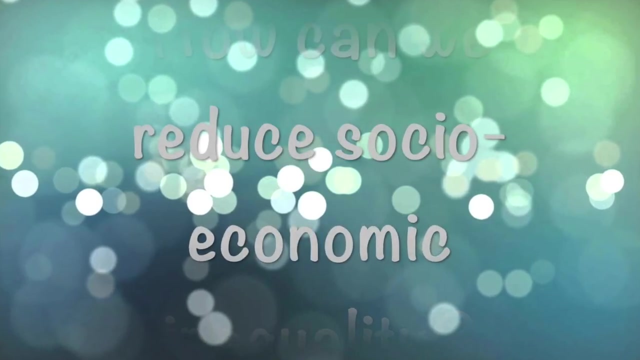 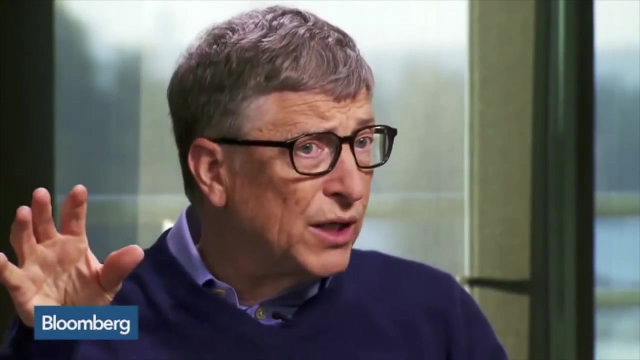 It's the result of policy decisions on taxes, education, trade, labor, macroeconomics and financial regulation, all of which shifted economic power away from low- and moderate-income American families. I believe it's in a balance that you should have progressive taxation that as you get,